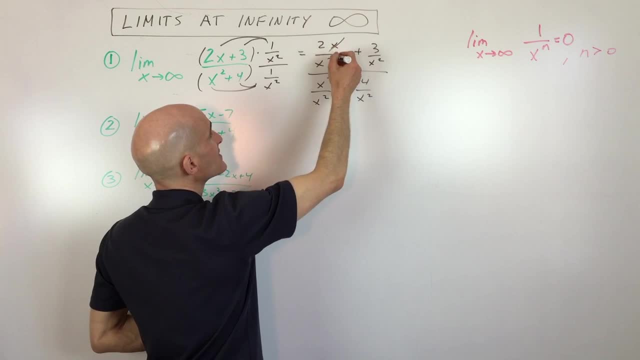 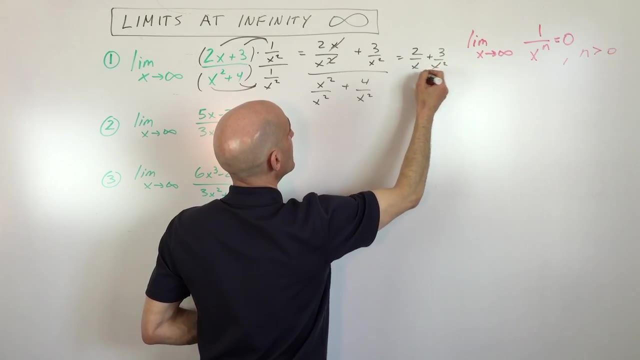 Okay. now, if we simplify this further, you can see one of these x's cancels with one of these. Okay, so we have 2x divided by x squared, 2 over x plus 3 over x squared. okay, And then x squared divided by x squared is 1,. 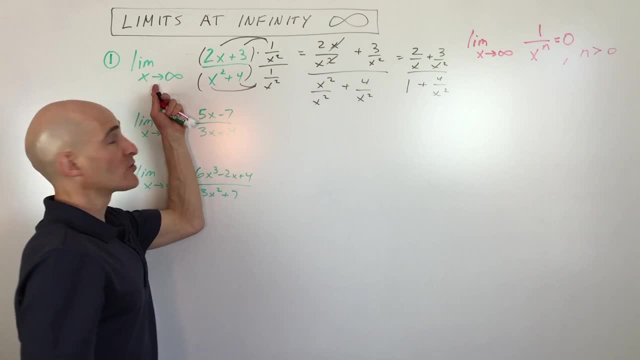 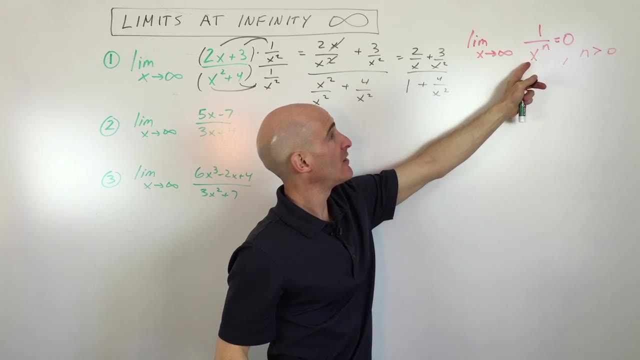 and we have 4 over x squared. Okay, now keep in mind we're doing the limit as x approaches infinity. but notice what happens. So when the numerator is a constant, okay, and the denominator has a variable, okay, and it's raised to a positive exponent, like we have here: x to the 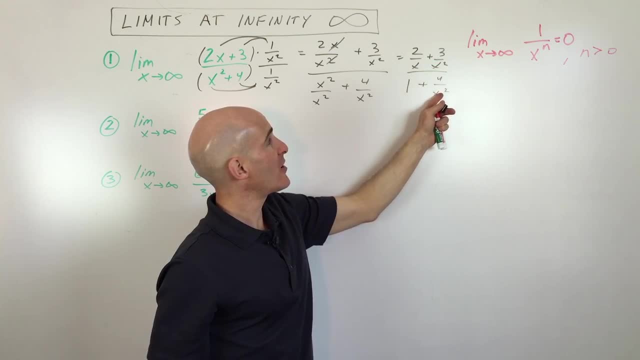 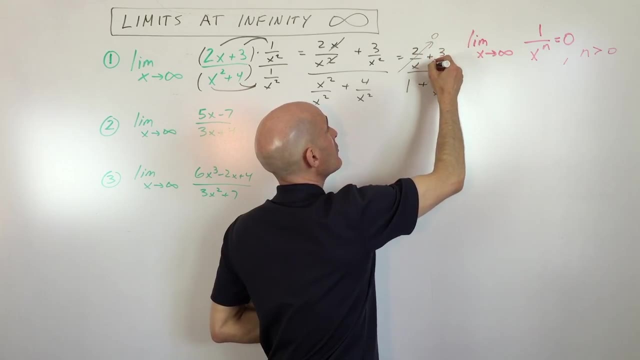 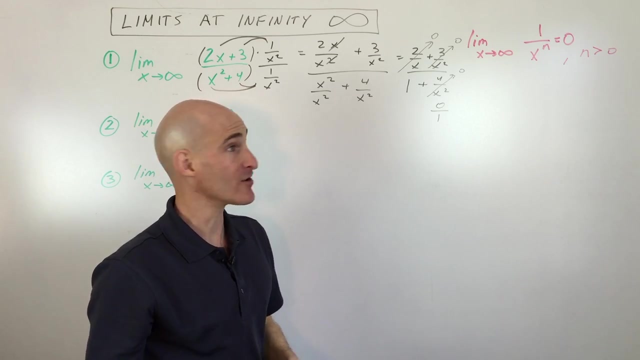 first, x squared. x squared as x gets larger and larger because the numerator is staying constant. it's going to get smaller and smaller. It's going to approach 0. So I'm just going to go like this, I'm going to say 0,, 0,, 0.. So what we have is 0 divided by 1.. 0 divided by 1 is 0.. So the limit. 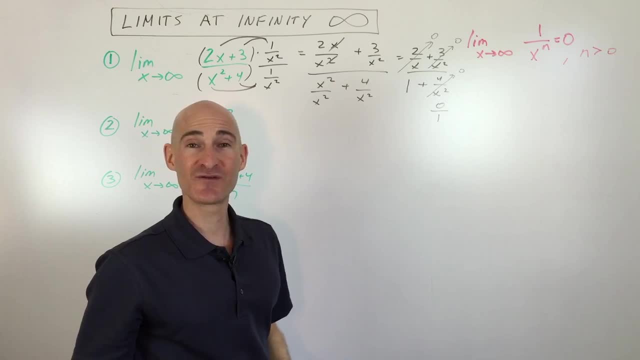 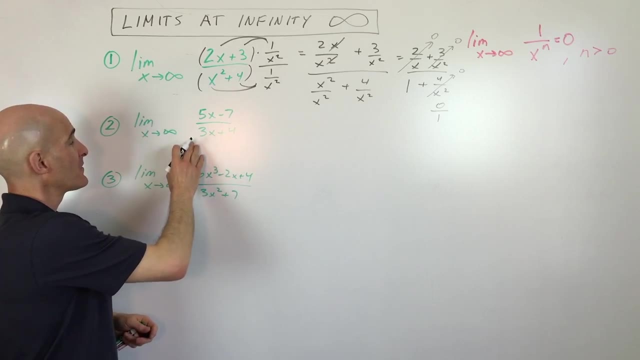 of this whole quantity is just going to be 0 as x approaches infinity. So are you with me? so far, All right, let's take a look at another example. Let's take the intuitive approach first. So this one. what do you think the limit is as x gets larger and larger. 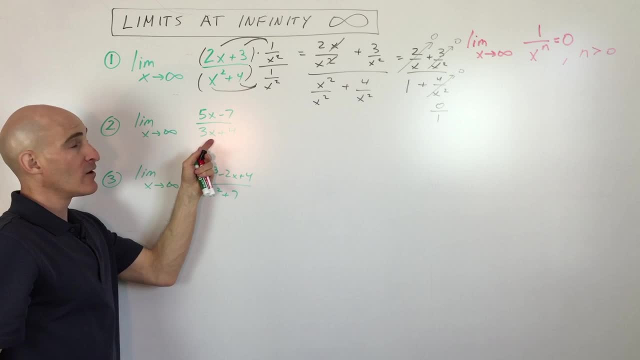 So take a second. What do you think happens there? Okay, if you guessed that it's five-thirds, you're right. Okay, and let's see how we came about that. See, as x gets larger and larger, does 7 change? Does 4 change? No, those are constants, They stay. 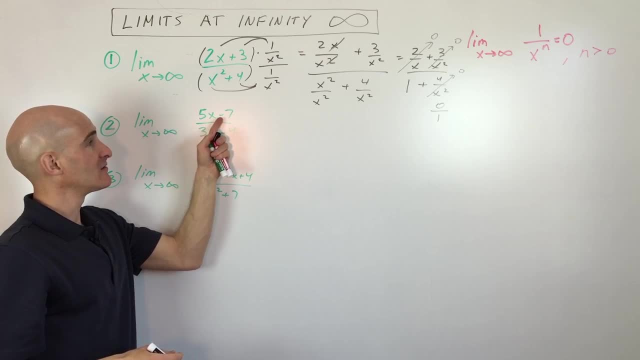 the same right. So what happens is: if x is 1,000, you know, you're just taking away 7.. If x is a million, you're just taking away 7.. So this term here is far outpacing this constant, The constant. 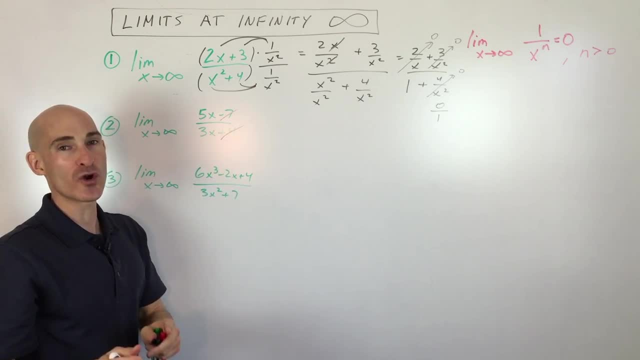 doesn't change like that. So we can essentially ignore that, because as x gets larger and larger, it's like if I told you I'm going to give you a million dollars times 5, but then I said, okay, but you have to give me back. 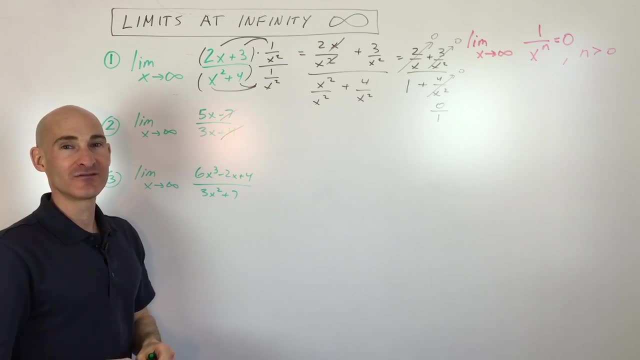 $7, see minus 7.. You'd say: oh, you know, it's no big deal, right, It's still approximately $5 million, right, Okay? so same thing here. okay, If I give you $3 million, right, 3 times a million. 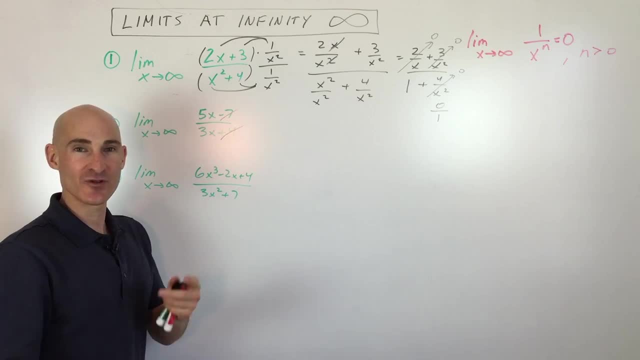 and then I say, oh, I forgot to give you 4 more. you'd say, oh, don't worry about it, because 3 million, 3 million, 4, it's about the same right. So we're zeroing in on this quantity right here. Notice that the x's, they're going to cancel one. 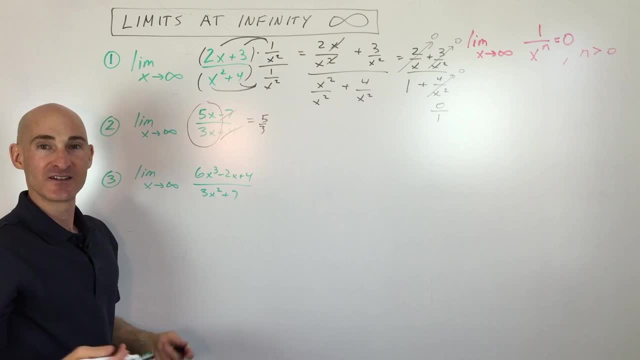 another out. So this is just going to be 5 thirds. So that's it. Okay. now, if you want to do this in a more rigorous fashion, we're going to do just like we did here: We're going to take the highest. 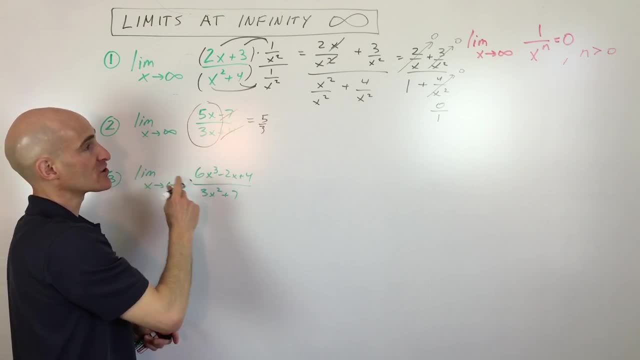 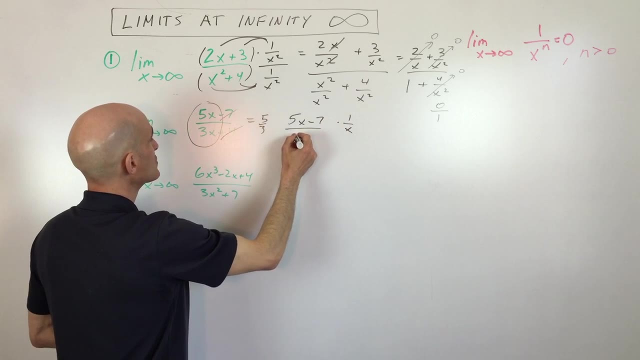 degree power of x, which is x to the first, and we're going to multiply the numerator and the denominators, okay, by 1 over x. okay, So I'm going to do the same thing to the numerator and denominator, because this is like multiplying by 1.. So I'm going to do the same thing to the 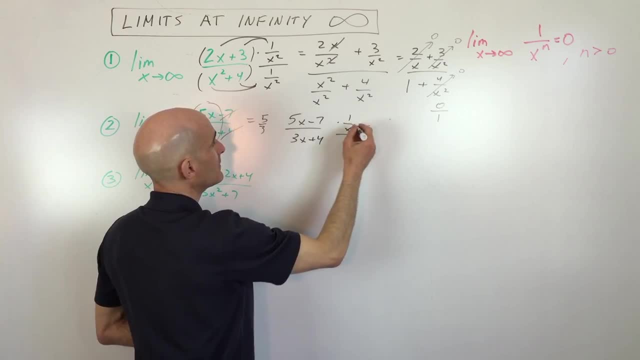 denominator and if I distribute it to each of these terms, what do I get? I get this would just be 5,, this is going to be 7 over x, this is going to be 3, and this is going to be 4 over x. But 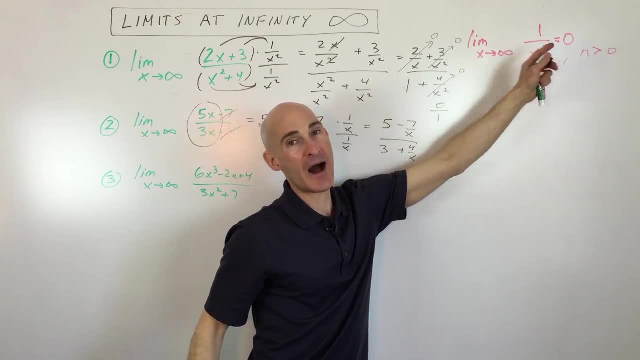 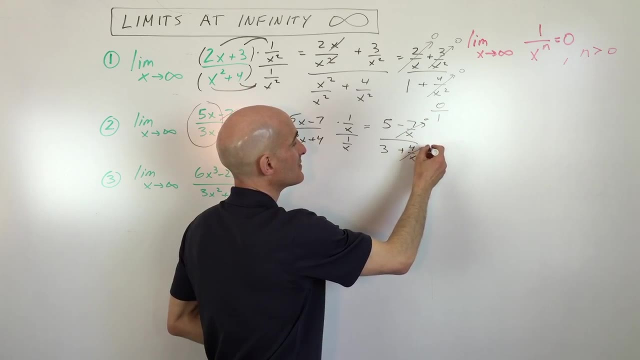 just like we talked about over here. if you have a constant in the numerator and x to a positive exponent as x gets larger and larger, this whole thing is going to go to well. this quantity is going to go to 0,, this quantity is going to be 0, and we're going to be just left with 5 over 3.. 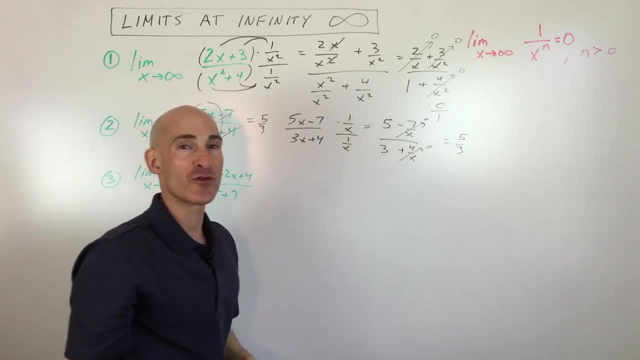 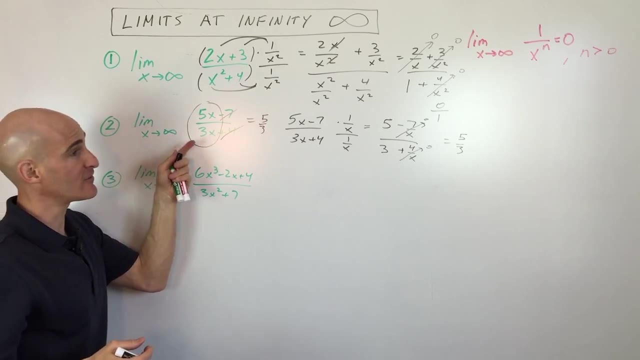 So the limit is 5 thirds Before we go further. you're probably thinking what happens if we're going to negative infinity. So let's say, instead of the limit as x approaches positive infinity, meaning, as we're going to the right on the graph, we go to the left on the graph. you know all the way to the left Well, 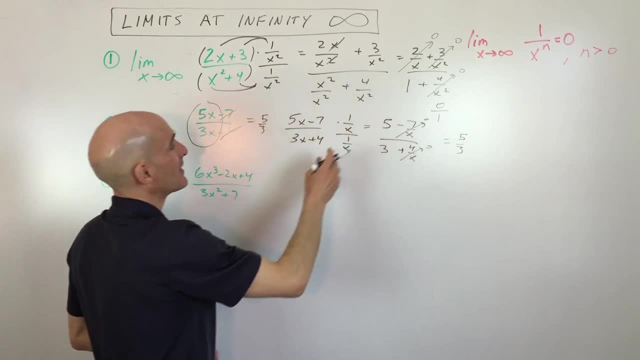 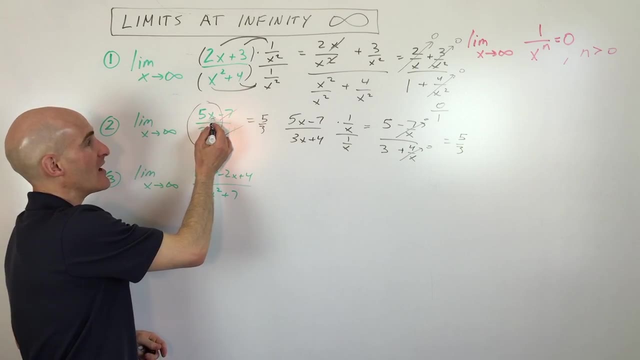 still for this one. you're still going to get 5 thirds. okay, Because you can see, if this was like, these are canceling out right. These are insignificant, right. Even if this was a negative 1 million, okay, x is getting a really large negative now and this is a. 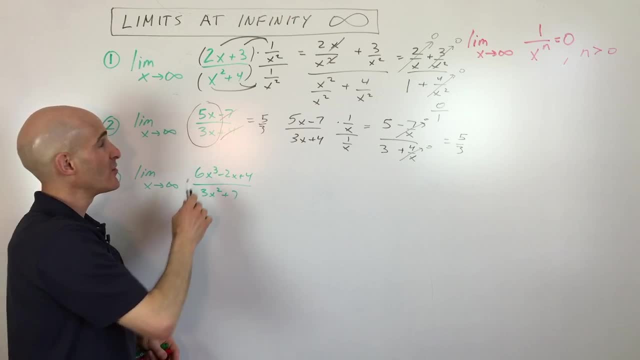 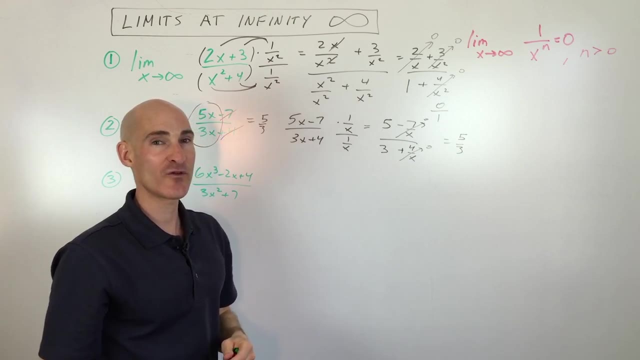 negative 1 million, you're going to have negative 5 million divided by negative 3 million. The two negatives are going to cancel and you're still going to get this ratio: 5 thirds. okay, So you're with me so far. Let's look at one last example. okay, This is like the third scenario here. So 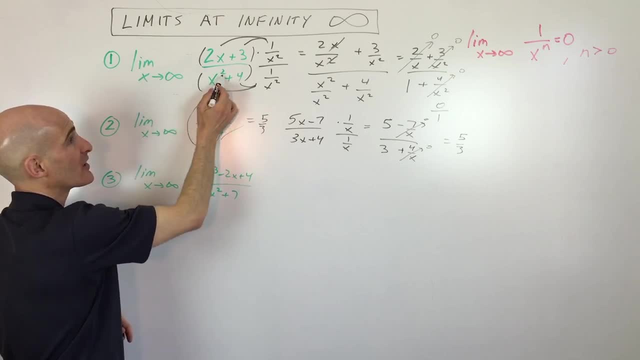 this one we had. the denominator's highest power term- okay, is greater than the numerator's highest power term. That went to 0,. okay, That limit was 0. This one, it was a tie, okay, So even if I. 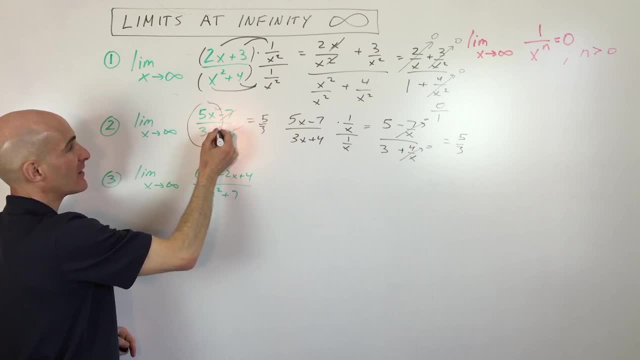 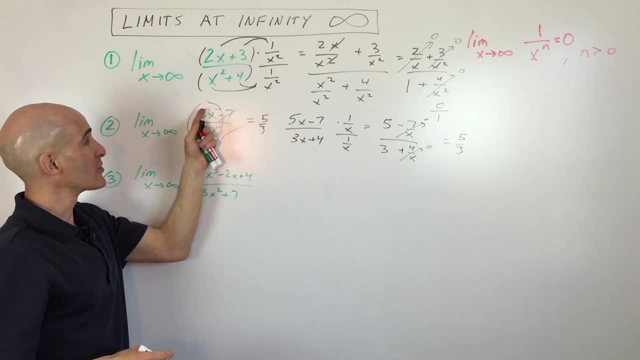 okay, the same highest powered terms. those are the same. you're going to get the ratio of the coefficients in front of those highest powered terms. Now, the third scenario here is where the numerator's highest agreed term- okay, that's this one here- is to a higher power than the denominator's. 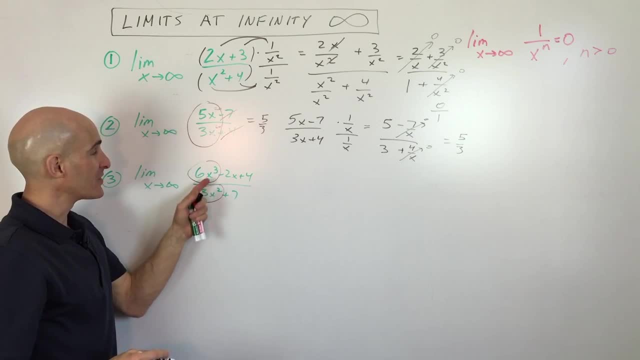 highest powered term. okay, So what that means is that this numerator is growing at a much faster power. okay, So this denominator x is going to tend to outpace whatever the denominator's highest powered term is right, And we know that this one will get smaller at a much faster. 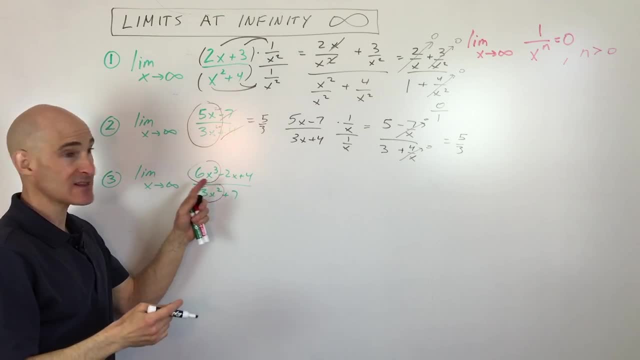 power than the denominator. we know that that denominator can get even bigger in here. So this time we're literally breaking the denominator right and we're not going to be able to bark back. okay, This denominator. here it starts six. we're not good at this one, We're going. 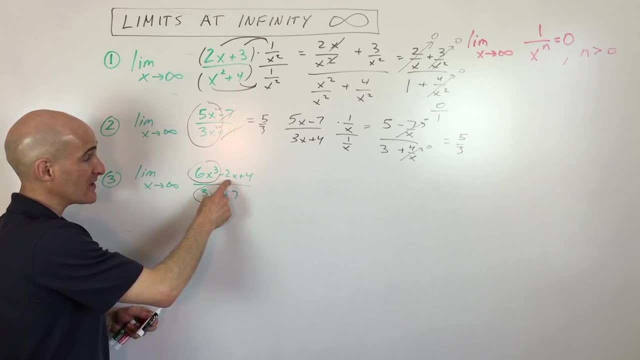 to have every step of the way around, in terms of what our denominator's highest or lowest power takes. See, this is not having very much impact, you know, on the overall value of the numerator, like this term is. So we can, essentially, as x gets larger and larger, we can ignore these terms because you know they're not adding very much influence. okay, 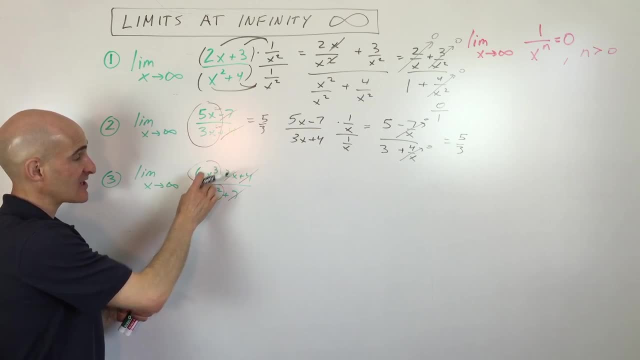 So this reduces down in essence to 6x cubed to 3x squared, And if we reduce it down even further, we get 2x, See 6 divided by 3 and x cubed divided by x squared. 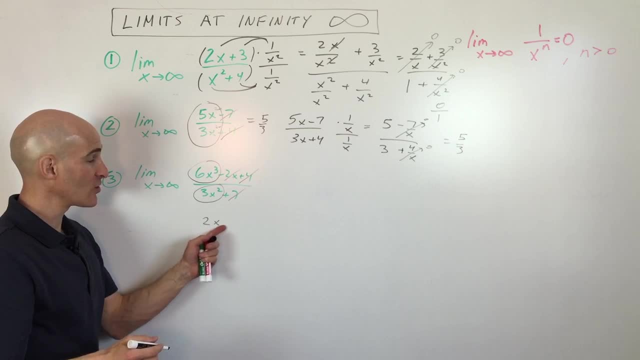 So now you can see, as x approaches infinity, this is going to go to 2 times infinity, right? It's going to go up to infinity, right, like that. Now, if x is approaching negative infinity, you're going to the left on the graph. then this would go to negative infinity, okay. 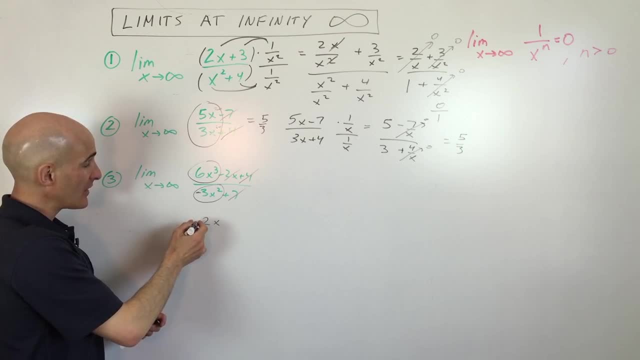 Now, if I change this up a little bit, if I make this a negative, okay, then this would be like negative 2x, As x gets larger and larger. this would actually go down, down, down towards negative infinity. But if you're going to negative infinity, the two negatives would cancel.